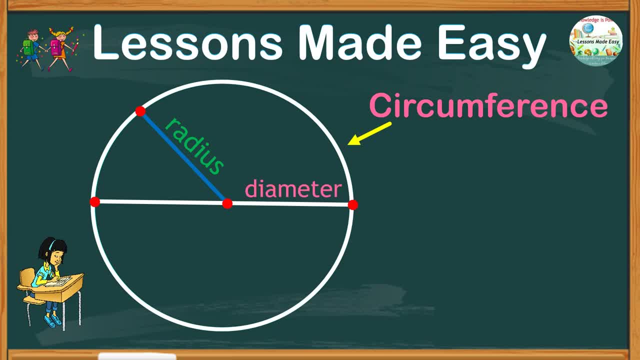 the circle is called the radius. The line segment that passes through the center and whose end points lie on the circle is called the diameter. The diameter is twice or two times the radius. If the radius is four meters, double this number means the diameter is eight meters. Therefore, the radius is only half of the diameter, or radius equals diameter divided by two. But how do we calculate for the circumference? Do you have any idea? 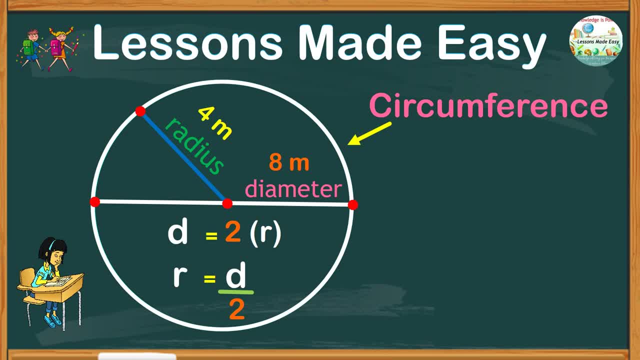 To calculate the circumference we must at least have the measurement of either the radius or the diameter. Although we can estimate the circumference, it is approximately three times the diameter. This is just an estimation, but if we measure it very carefully you'll find it's about. 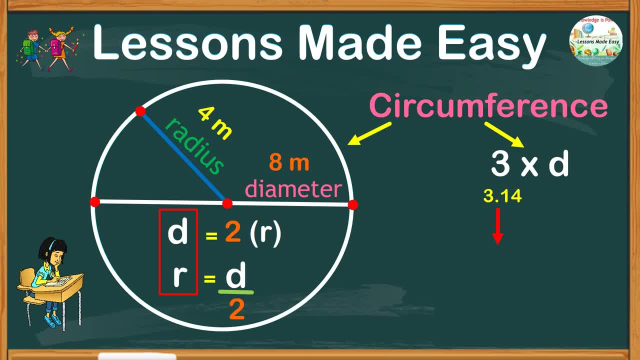 3.14, which is represented by the Greek symbol pi. In other words, circumference, can be calculated by taking the value of pi times the diameter, or c equals pi d. In some cases, the given measurement is the radius. For this we can use the formula 2 pi r. It is actually the same, because this 2r, or two times the radius, is derived from d, which is the diameter. To further understand this concept, let's try to answer a few questions. 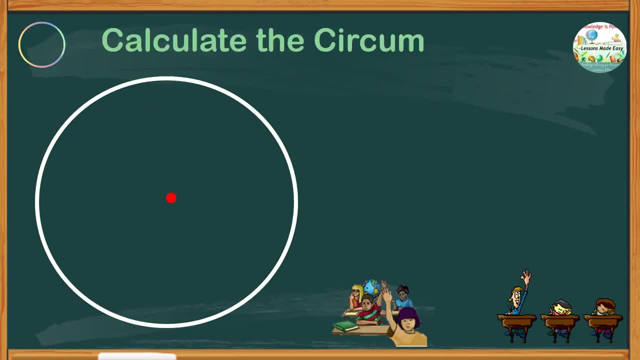 Try to calculate the circumference of a circle with a diameter of 20 centimeters. Previously, we studied two ways to find the circumference. One is circumference equals pi d and the other is circumference equals 2 pi r. Which one of these should you use? 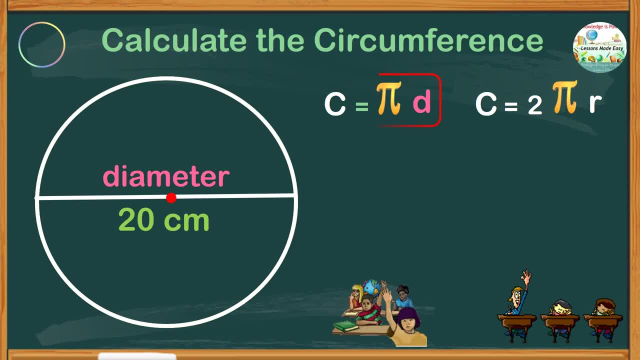 For this problem it is reasonable to use c equals pi d, since the given measurement is the diameter. It is unwise if you use 2 pi r, because using this formula means you have to divide the diameter by 2 to get the radius and then multiply by 2.. 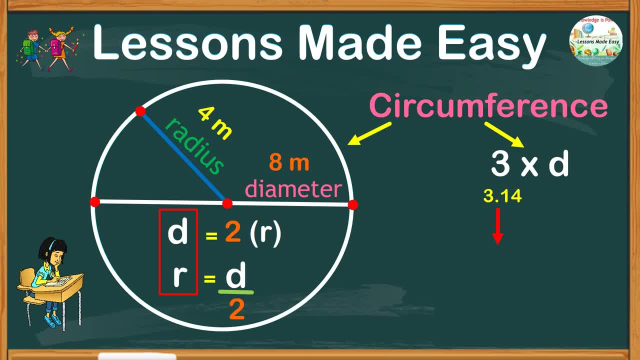 3.14, which is represented by the Greek symbol pi. In other words, circumference, can be calculated by taking the value of pi times the diameter, or c equals pi d. In some cases, the given measurement is the radius. For this we can use the formula 2 pi r. It is actually the same, because this 2r, or two times the radius, is derived from d, which is the diameter. To further understand this concept, let's try to answer a few questions. 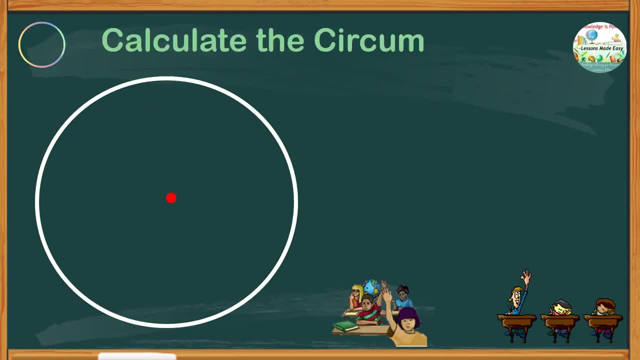 Try to calculate the circumference of a circle with a diameter of 20 centimeters. Previously, we studied two ways to find the circumference. One is circumference equals pi d and the other is circumference equals 2 pi r. Which one of these should you use? 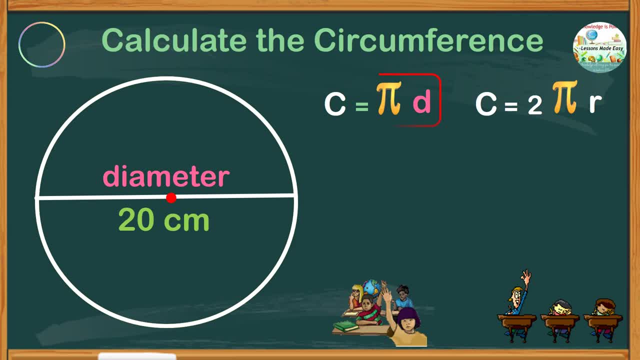 For this problem it is reasonable to use c equals pi d, since the given measurement is the diameter. It is unwise if you use 2 pi r, because using this formula means you have to divide the diameter by 2 to get the radius and then multiply by 2.. 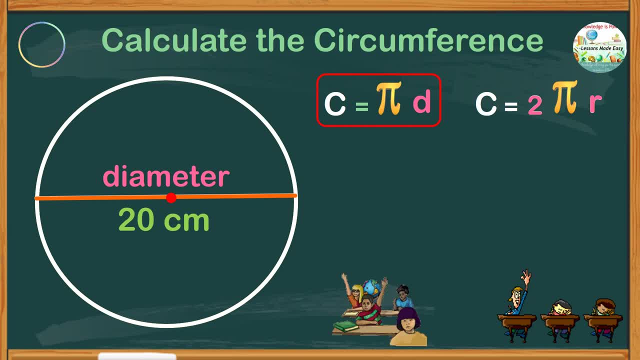 This is just a waste of time, so let's stick with pi. d Circumference equals pi. Let's substitute the value of pi, which is 3.14, times the diameter, which is 20 centimeters. If we multiply 3.14 by 20,, we get 62.8.. So our circumference is 62.8 centimeters. 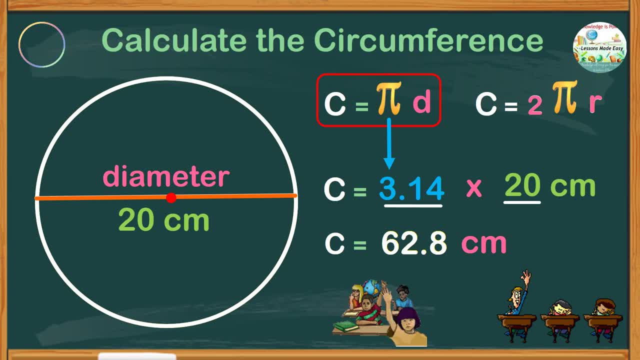 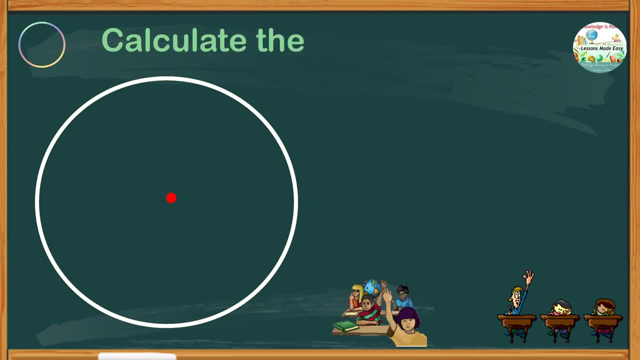 By the way, I have created a video about multiplication. If you're interested, you can check the link in the description box. Alright, then let's proceed. How do you calculate the circumference when the given measurement is a radius of 12 centimeters? 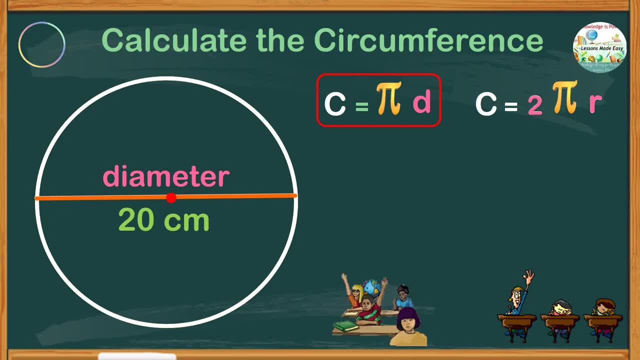 This is just a waste of time, so let's stick with pi. d Circumference equals pi. Let's substitute the value of pi, which is 3.14, times the diameter, which is 20 centimeters. If we multiply 3.14 by 20,, we get 62.8.. So our circumference is 62.8 centimeters. 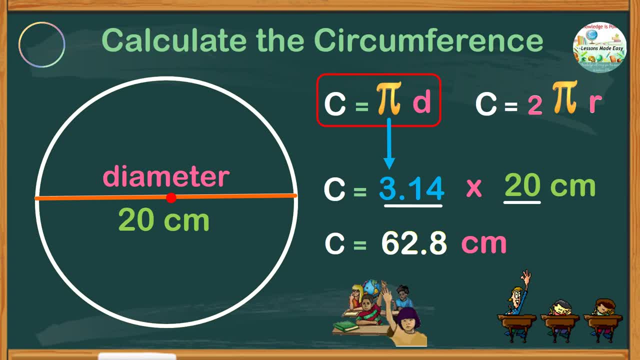 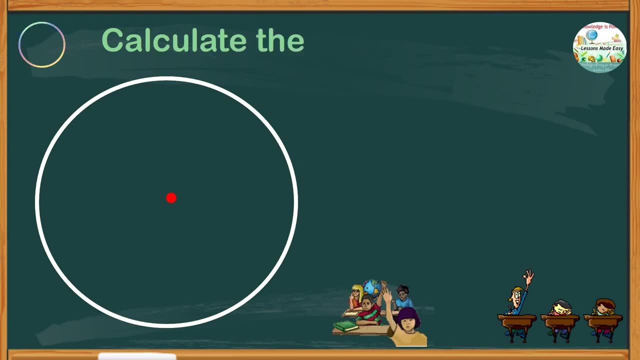 By the way, I have created a video about multiplication. If you're interested, you can check the link in the description box. Alright, then let's proceed. How do you calculate the circumference when the given measurement is a radius of 12 centimeters? 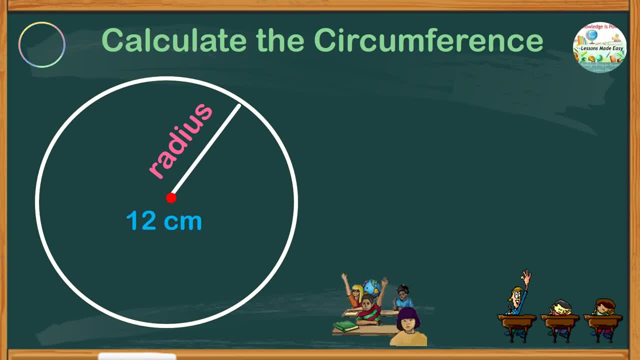 Given the radius, we can use the formula: circumference equals 2 pi r. Just substitute the values We have. c equals 2 times the value of pi, which is 3.14, times the given radius of 12 cm. Because we have 3 given quantities, we have to multiply. the first two numbers, which is very small: 2 times 3.14 times the given number, which isかnon fillestan prime. So what we need to do is to multiply the covering number of 4 by the given number, 2 times 3.14 times the given number, And we will see that the number 2 and the given number will be equal to 3.. 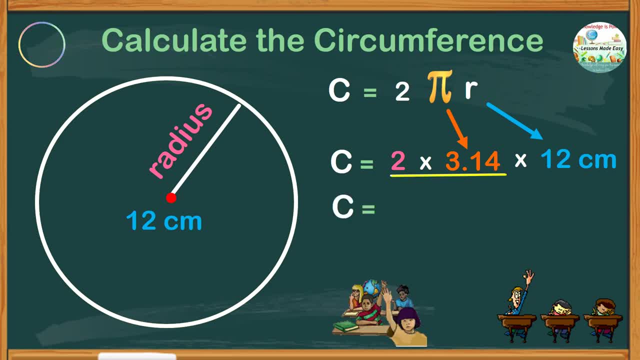 Let's start with the form. There are these three values here. that are two nice numbers. So then that has to fit into our problem statement. So just that the求 is at the fundamentally correct answer, 3.14 would give us 6.28.. And then multiply this number by 12.. We get a product of 75.36.. 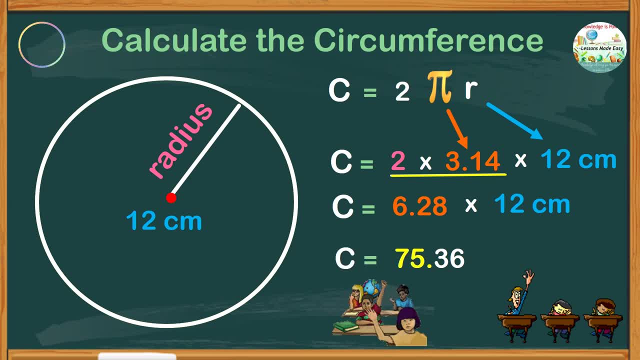 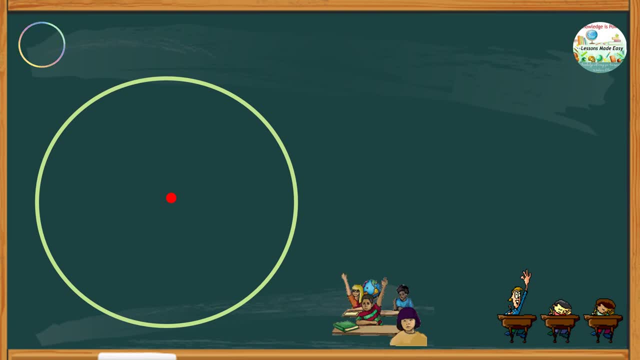 So the circumference is 75.36 centimeters. But how about if the circumference is already given? How do you calculate the diameter? Try this one: Calculate the diameter of a circle with a circumference of 78.5 centimeters. To find the diameter, we can still use the formula C equals. 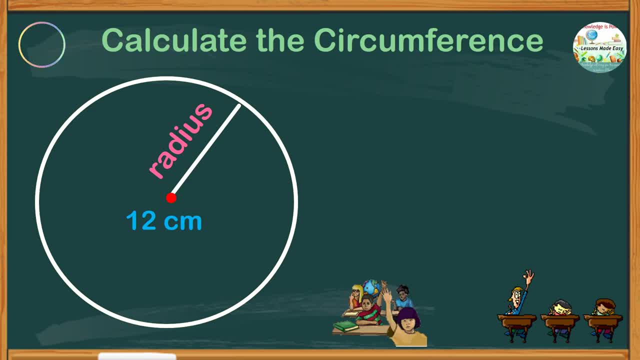 Given the radius. we can use the formula: circumference equals 2 pi r. Just substitute the values We have. c equals 2 times the value of pi, which is 3.14, times the given radius of 12 cm. Because we have 3 given quantities, we have to multiply the first two numbers, which is very 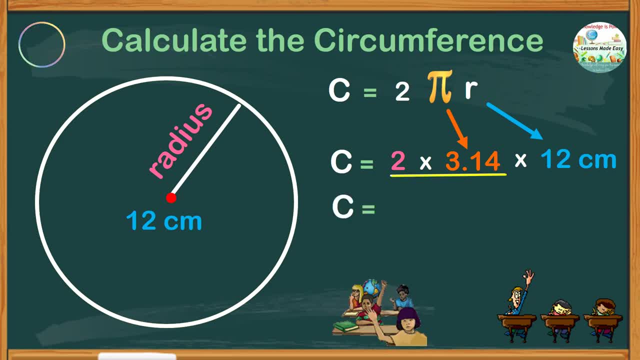 small, 2 times 3.14.. So we have 3.14 times the value of pi, which is 3.14, times the given radius of 12 cm. So the circumference of this circumference is 75 cm. The circumference of the other circumference is 75.36 cm. 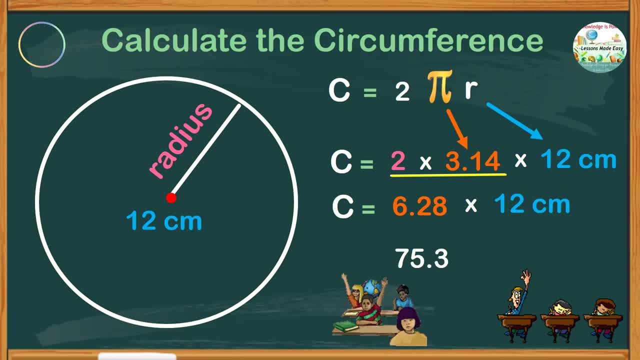 We have to multiply the Earth's diameter, which is 3.14, times the given radius of 12 cm, which is 5.24 cm. So we have 2 pi r. This time we multiply the circumference and we get 2 pi r, which is: 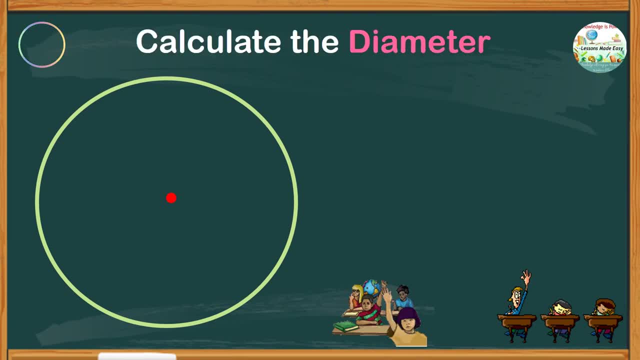 6.28 cm. So we have 2 pi r times 3.14.. This is very small, 2 pi r. This is also 3.24 cm. So the circumference of this circumference is 75 cm. Calculate the diameter of a circle with a circumference of 78.5 centimeters. 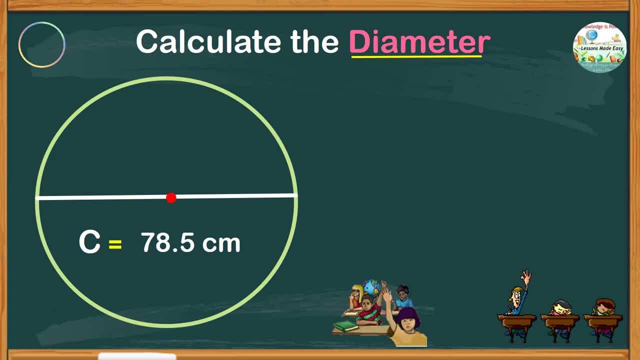 To find the diameter, we can still use the formula C equals pi- D. All we have to do is substitute the values- The circumference is 78.5 centimeters, equals pi, which is 3.14,, and keep D as it is. 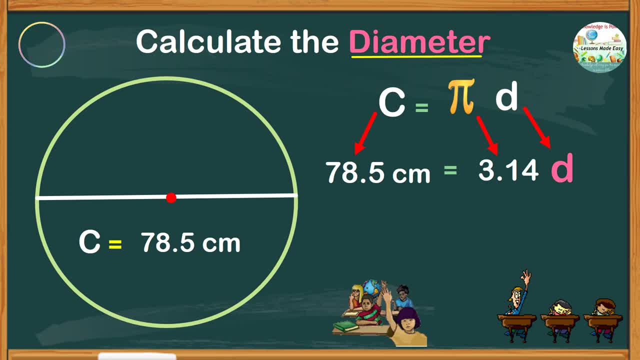 So, to find the diameter, we may transpose or move pi to the other side of the equation if you prefer to do so. But I guess it is much easier to understand if we keep the equation as it is and do the simple steps. Since we only need the diameter, we might as well get rid of pi. 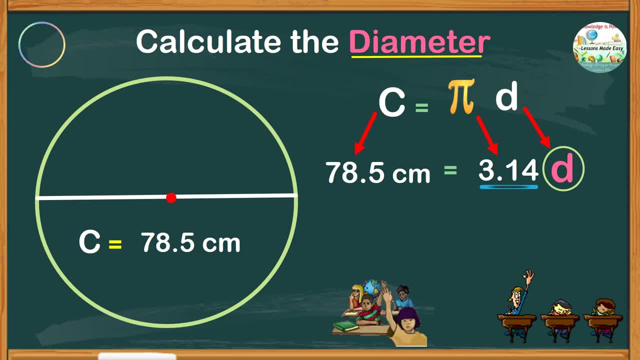 But how do we do it? Just by dividing pi with the same value of 3.14. And we get 1, which we don't need actually to write, or just simply cancel it. In short, what's left is the diameter. 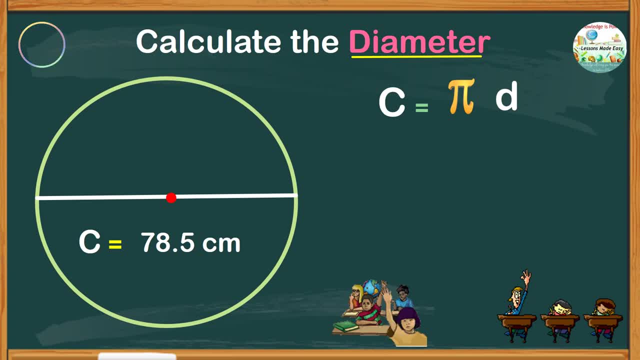 pi d. All we have to do is substitute the values- The circumference is 78.5 centimeters equals pi d- And then multiply this number by 12. We get a product of 75.36.. And then multiply this pi, which is 3.14, and keep d as it is, So to find the diameter we may transpose or move. 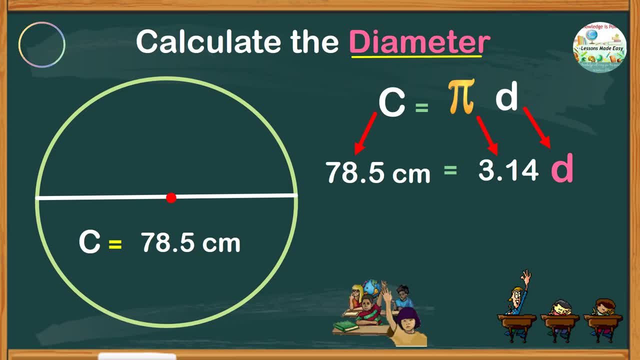 pi to the other side of the equation if you prefer to do so. But I guess it is much easier to understand if we keep the equation as it is And do the simple steps. Since we only need the diameter, we might as well get rid of pi. But how do we do it? We can use the formula C equals. 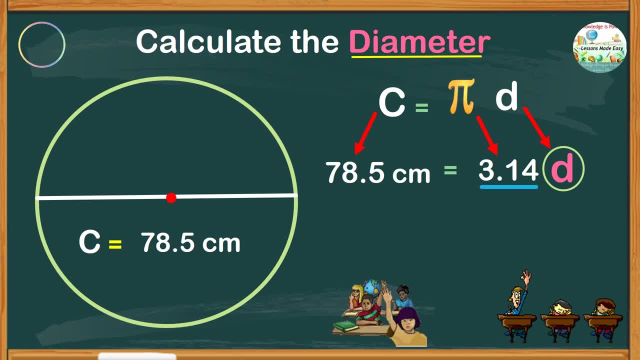 pi d Just by dividing pi with the same value of 3.14.. And we get 1, which you don't need to write or just simply cancel it. In short, what's left is the diameter Because we divide 3.14 on. 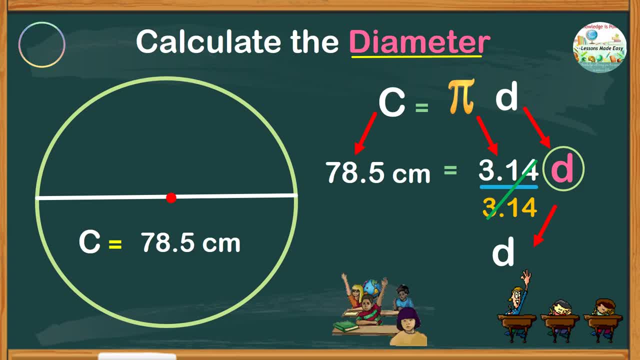 one side of the equation, we must also do the same on the other side. So divide the circumference by 3.14. And whatever the quotient is is our diameter. So we divide the circumference by 3.14.. So divide 78.5 by 3.14, we get a quotient of 25.. So our diameter is 25 centimeters. 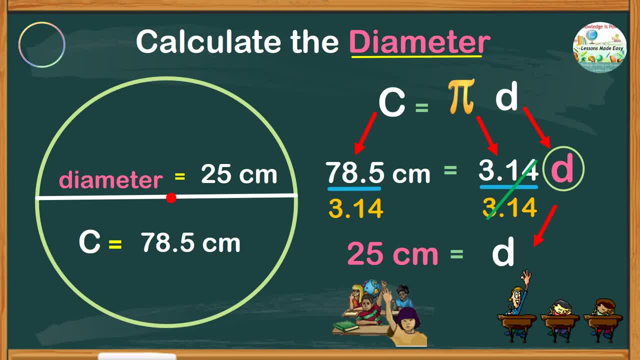 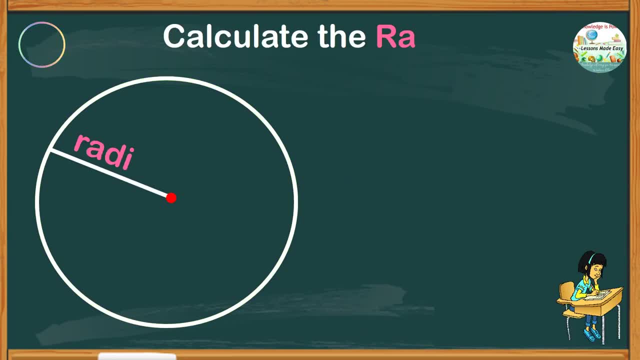 You can check out in the description box the link to a video on how to divide whole numbers and decimals. Let's try another one. Calculate the radius of a circle with a circumference of 94.5 centimeters And we get a quotient of 25.5 centimeters. So we divide the circumference by 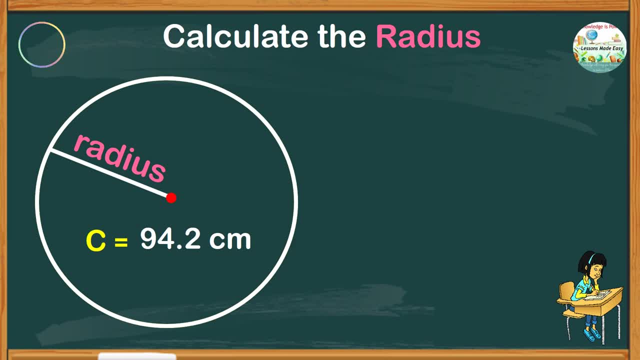 44.2 cm. In this problem we can use the formula C equals 2 pi r and substitute the values. The circumference is 94.2 centimeters equals 2 pi r. Let's make the number much smaller by dividing both sides of the equation by 2.. So what's left of the circumference is 47.1.. 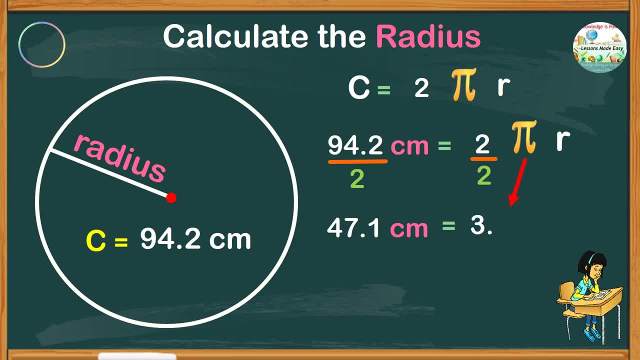 And on the other side of the equation we have a quotient of 2, pi, r. So we divide the circumference by 3.14.. And on the other side is pi, which is 3.14, and r. We need only the radius. So to get: